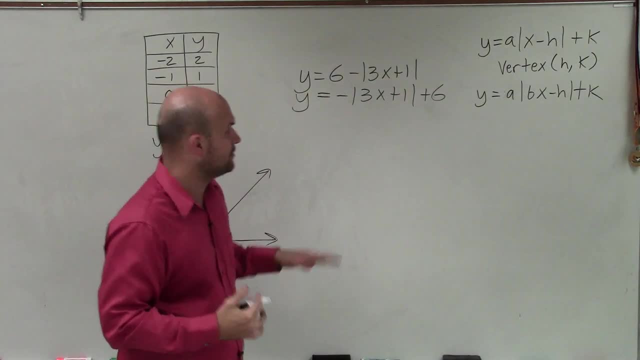 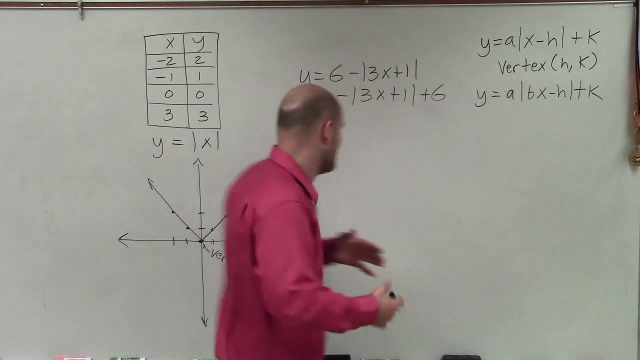 you see, I didn't write the vertex because there's a little bit of extra work we have to do. k is going to remain the same, So my k, my point 6, is still going to be my k. That means I'm going to take this graph and shift it up 6 units. Well, it's going to be reflected. 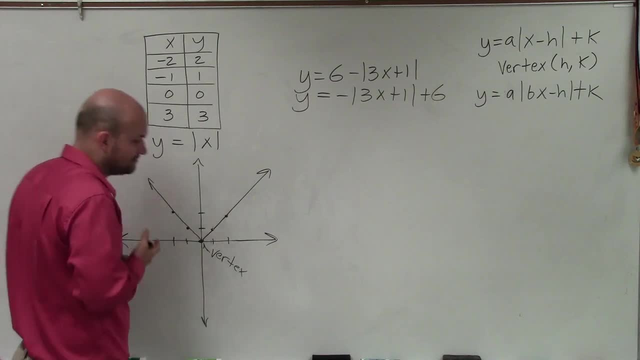 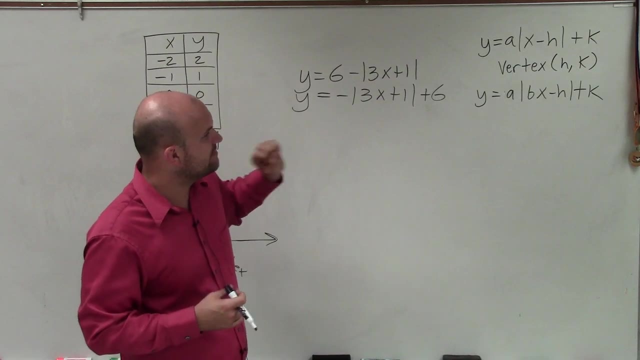 over the x-axis and then I'm going to shift it up 6 units, But what's important about this is identifying where I'm going to be shifting- left or right. So to do that, what you want to do is take whatever's in front of you, and you want to make sure that you. 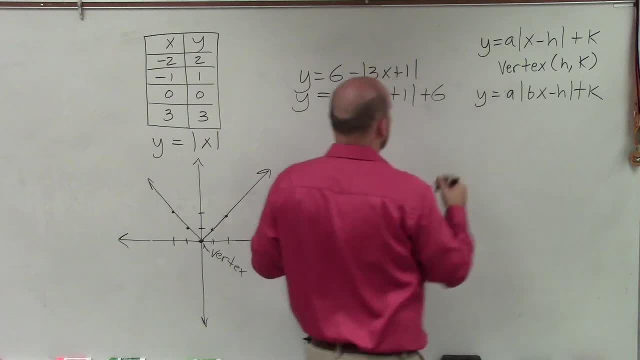 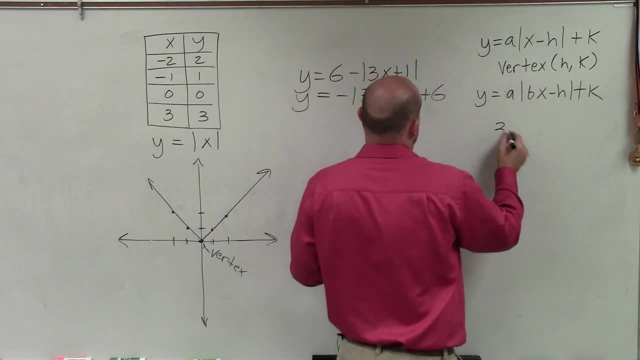 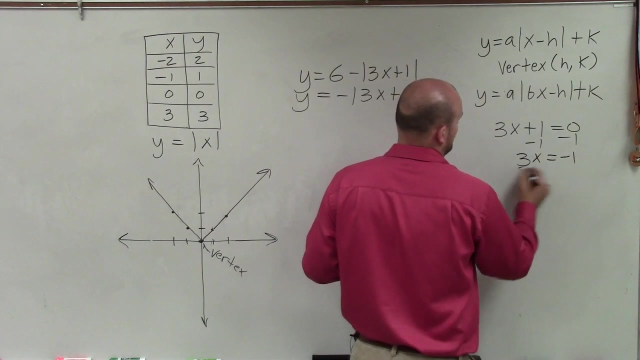 have whatever's inside your absolute value and set that equal to 0. That's going to be the new x-coordinate of your vertex, or what we call your h. So I take: 3x plus 1 equals 0.. Subtract 1, subtract 1.. 3x equals negative. 1. Divide by 3, divide by 3.. x equals a negative. 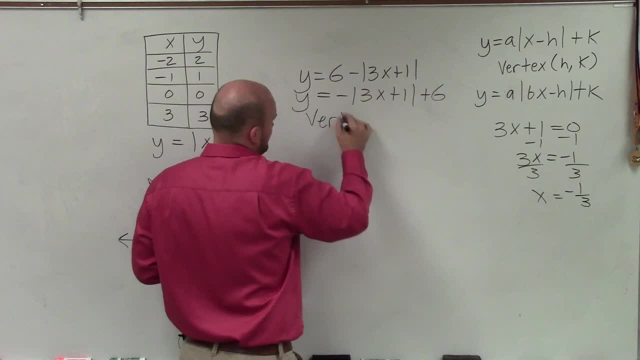 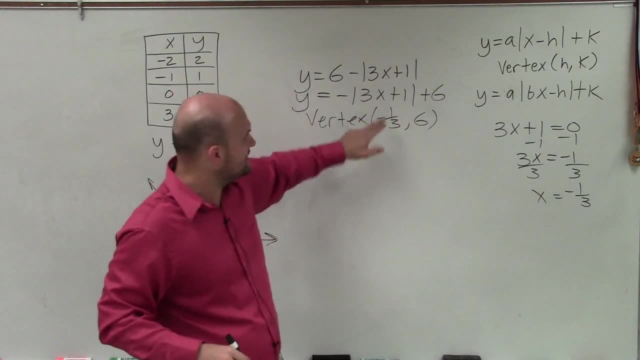 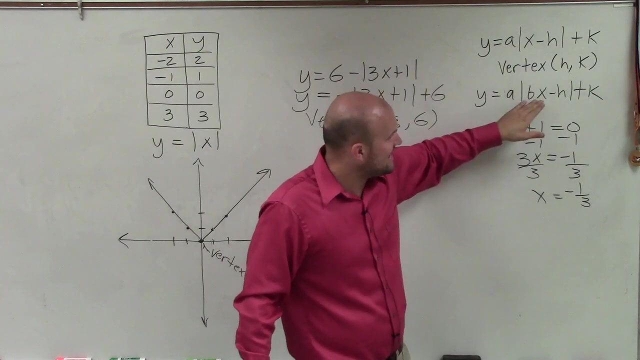 1 third. So now my new vertex is going to be negative 1, third comma 6.. All right, The k still remains the same, but my h is not just simply 1.. And that's the common mistake students make, Because, yes, when it's just x minus h, then it's h, But when it's bx minus, 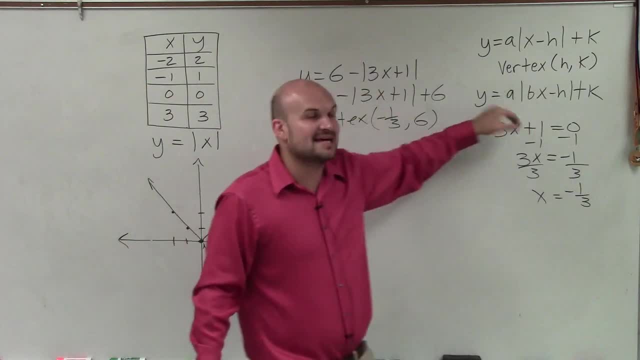 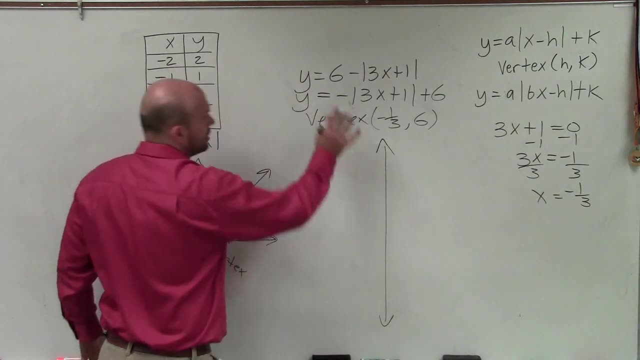 h. when there's that value that's being multiplied by x, you've got to set it in and solve to find your new value. So first thing I'm going to do is graph the transformations. We will go through how to graph the rest of it in just a second, But let's go through our new transformations. which would be a negative. So let's see: 1,, 2,, 3,, 4,, 5,, 6,, 7,, 8,, 9,, 10,, 11,, 12,, 12,, 13,, 13,, 14,. 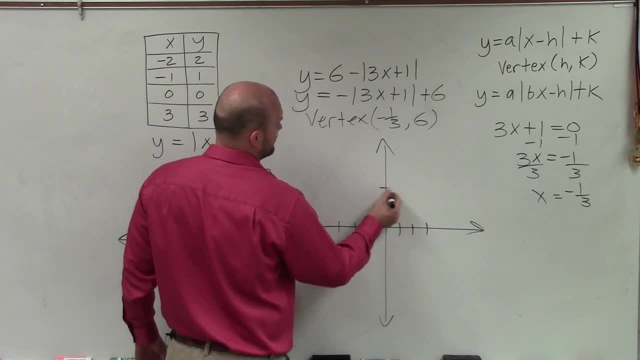 15,, 16,, 17,, 18,, 19,, 20,, 21,, 22,, 23.. 1, 2, 3.. And 1, 2,, 3,, 4,, 5, 6.. 1, 2,, 3,, 4,, 5, 6.. 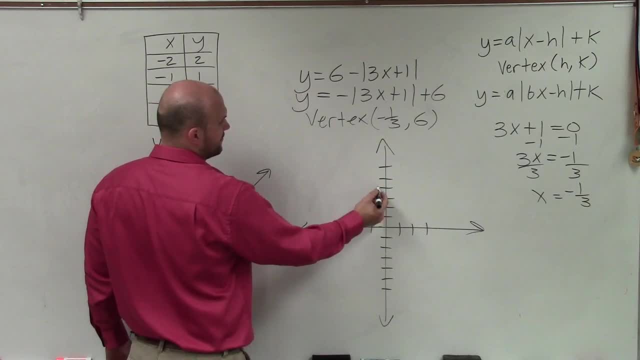 OK, So I'm going to go over negative 1 third up 6.. 1,, 2,, 3,, 4,, 5,, 6.. Now I know my graph is going to open down right, But I also know that I have fractions And a lot of times. 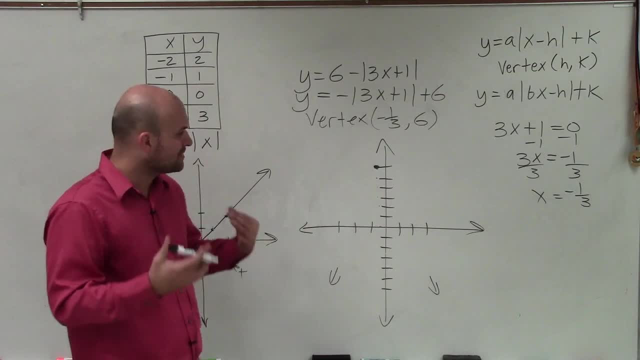 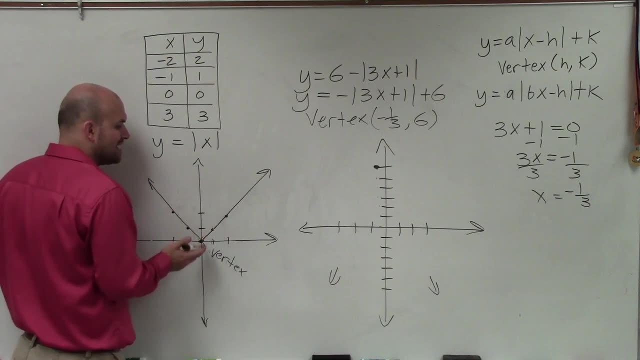 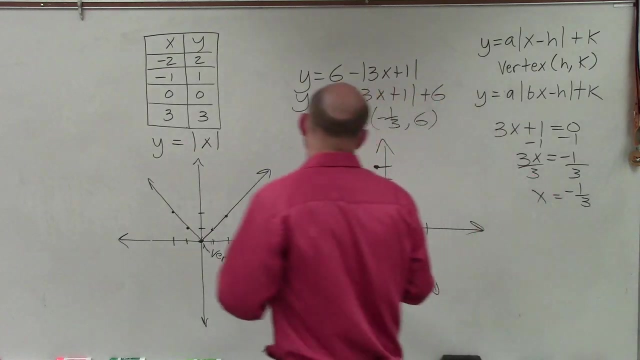 this can be pretty difficult or complicated, So remember that an absolute value equation has the axis of symmetry, And all we really need to do is just find two points that are on one side of the absolute value, Reflect them over. So what I'm going to do is I'm going to make a table of values And 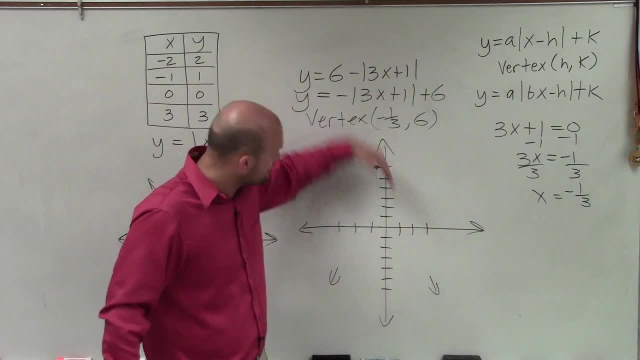 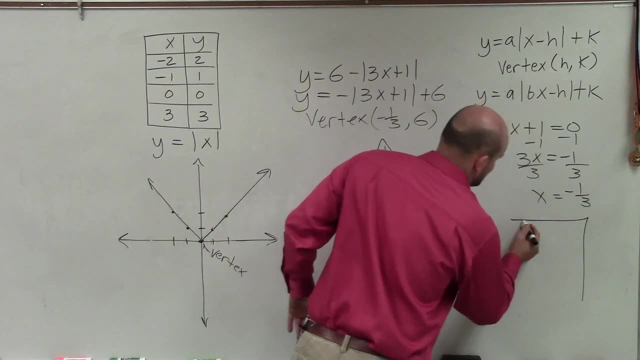 I'm going to make a table of values for the graph. that's going to go to the right And I know it's going to go down again because it's a negative right. I'm going to use two points. So I'm going to make a table here. That's a big table. We don't need that big. 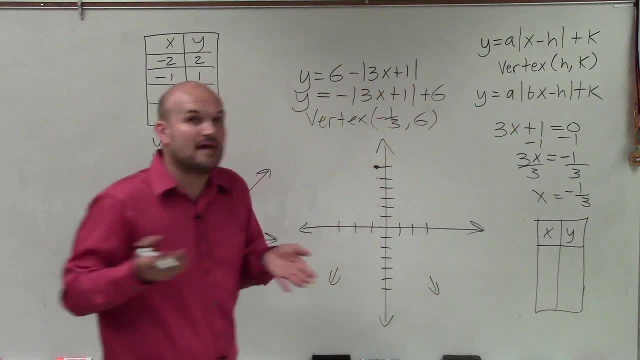 table x and y. I'm going to choose two values. Now you can be arbitrary to choose any two values for x and y, The two values. why don't we pick 0? That one's easy, And why don't? 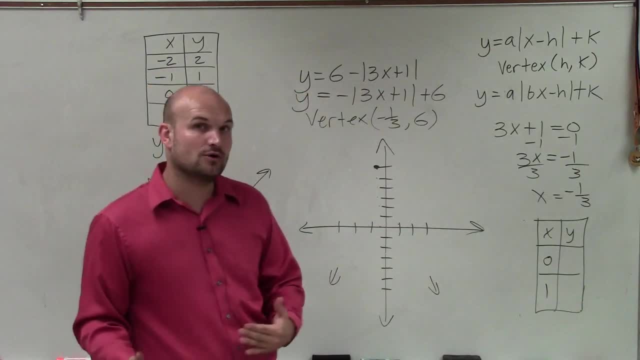 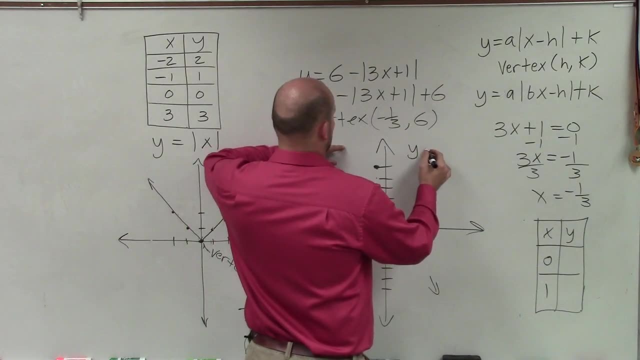 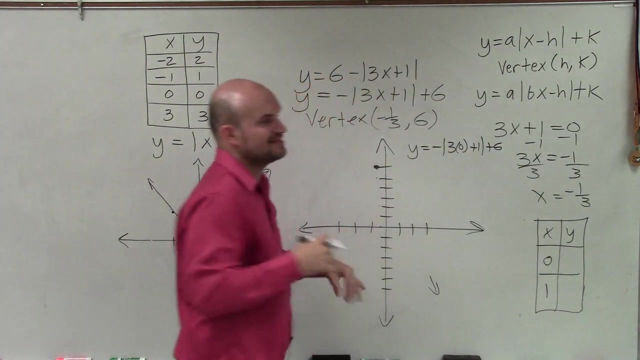 we pick 1?? That will be easy. Now to evaluate the y coordinate for those points, I'm just going to plug in 0 and 1 into my equation So I can have: y is equal to a negative absolute value of 3 times 0 plus 1 plus 6.. So now I'm going to say this out loud: 3 times 0 is 0. 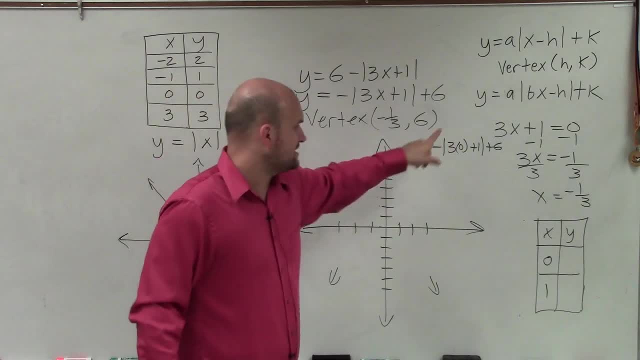 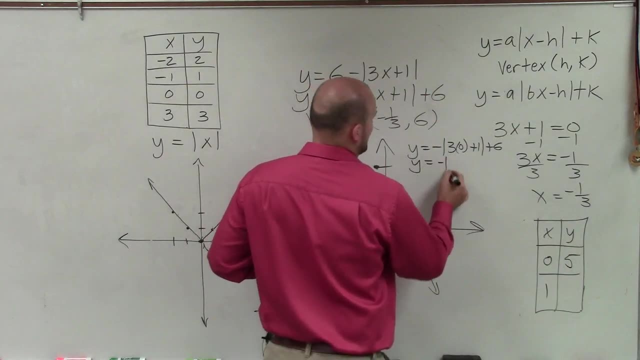 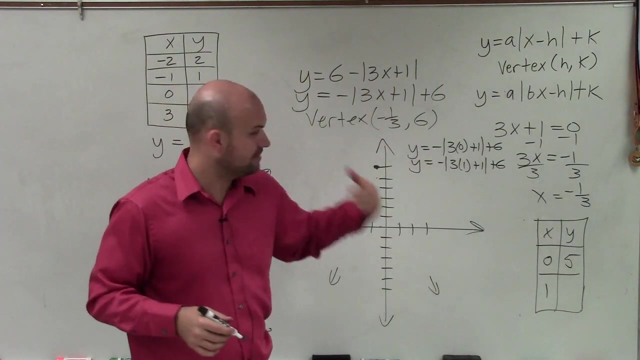 plus 1 is 1.. Absolute value of 1 is 1.. 1 times negative, 1 is negative. 1. Negative 1 plus 6 is 5.. Now let's do 1.. 1. y equals negative 3 times 1 plus 1 plus 6.. 3 times 1 is 3 plus 1 is 4. Absolute value. 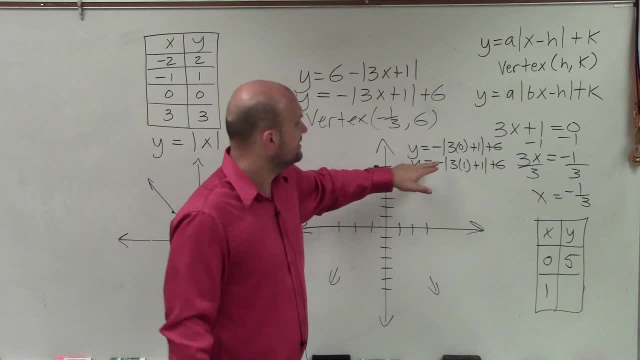 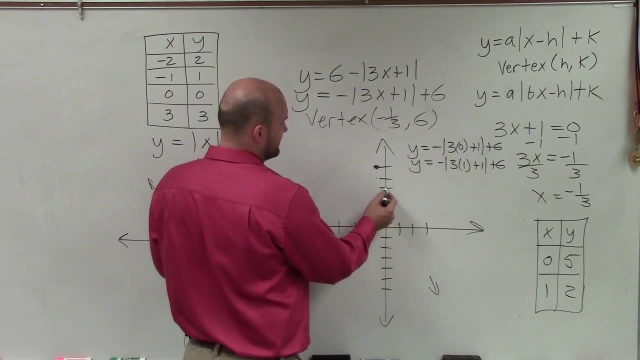 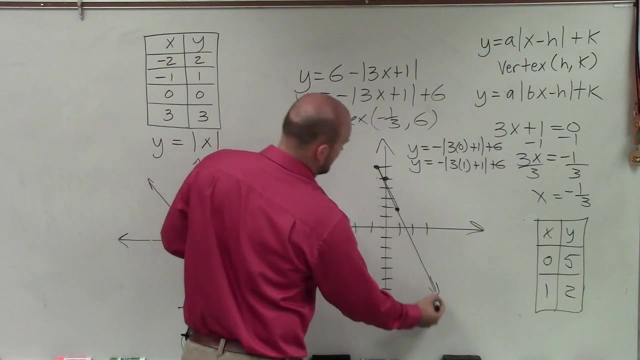 of 4 is 4 times negative. 1 is negative, 4. Negative 4 plus 6 is 2.. So therefore I can go over 0, 5.. So 1, 2,, 3,, 4, 5.. And then at 1, 2.. So you can see my graph goes down in. 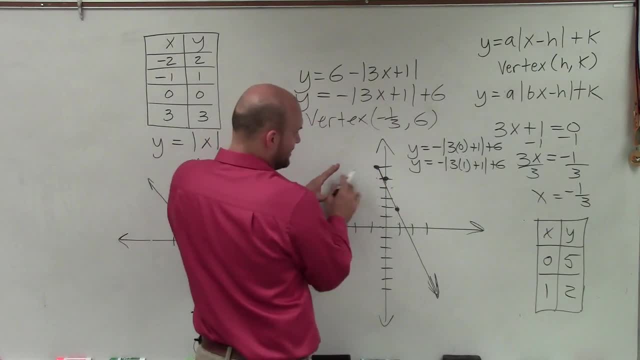 that direction, direction. Now, this is kind of a little difficult here. So this is at 1 third right, Well, at 0,. all I'm simply going to do is reflect this over. So I went from negative 1 third. 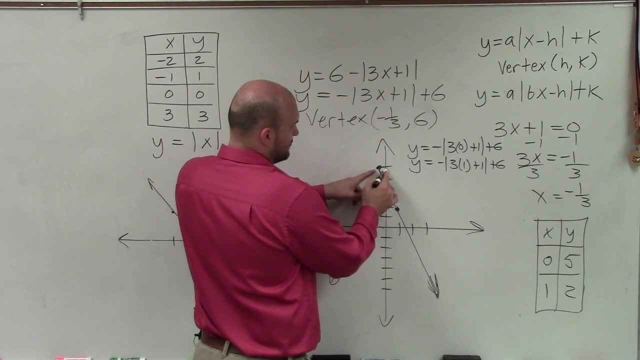 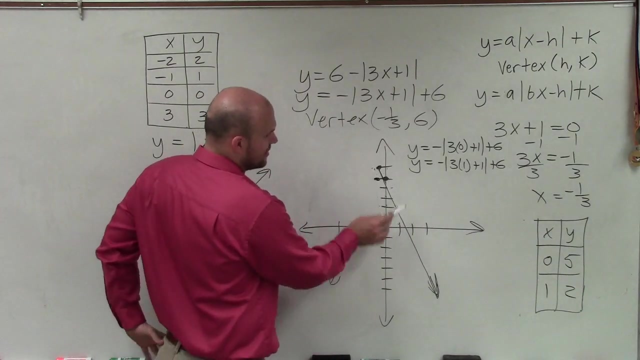 to 0 is a distance of 1 third. So I just need to go that exact same distance to the other side, which would be negative 2 thirds, and then go down to 6.. And then over here, the exact same thing. the distance from over 1 would be 1 and negative 1 third. So I'm going.